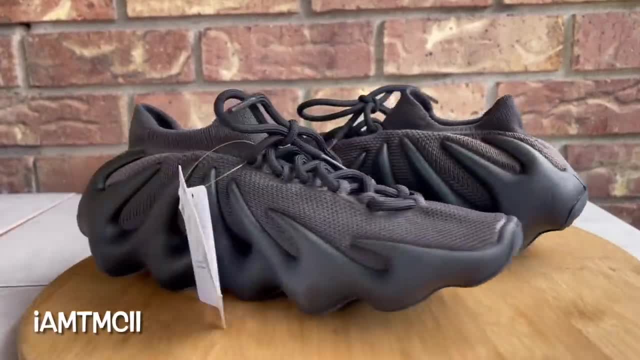 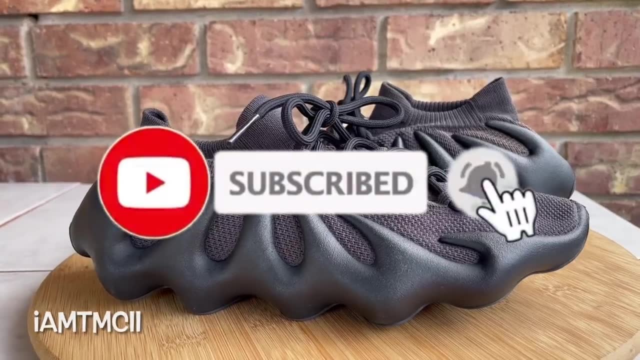 to the channel, Tell you thanks- mainly you know, thanks for taking out some time to drop by and check out one of my videos. While I have you here, do me a favor, Go ahead and hit that subscribe button and click that notification bell for me. That way, whenever I upload new material, post new. 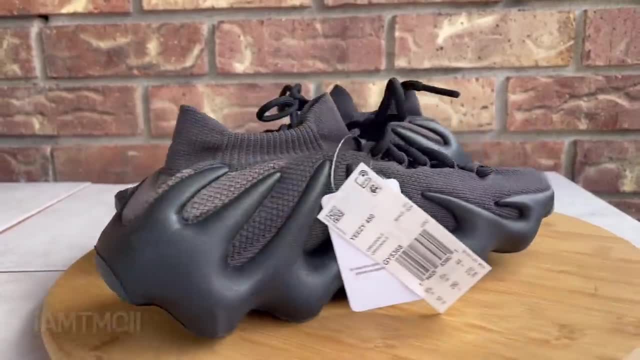 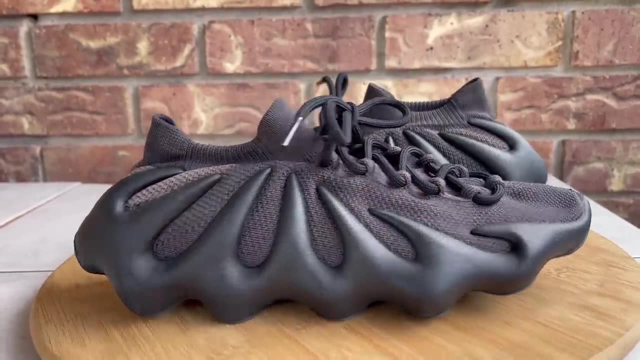 content or anything like that. you get notified, you can head to the channel and you can check out my latest video. You can also find me on Twitter and Instagram. My username is at imtmcii, So if you're on social media, go ahead and give me a follow there And, lastly, hit the thumbs up. That's. 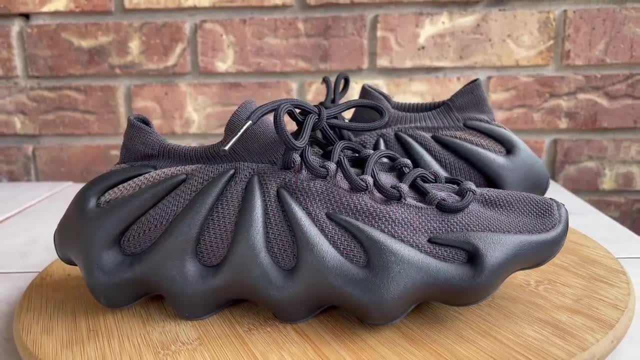 huge. That's major to me. It's an indicator Let me know that you guys enjoy the content, And it just kind of pushed me to keep on to record these videos whenever I'm out there. So I'm going to go ahead and hit that subscribe button and click that notification bell for me. 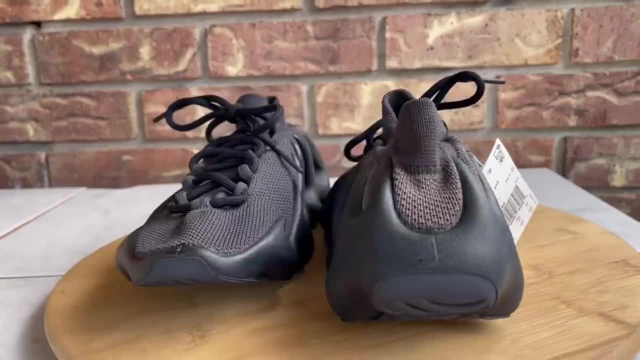 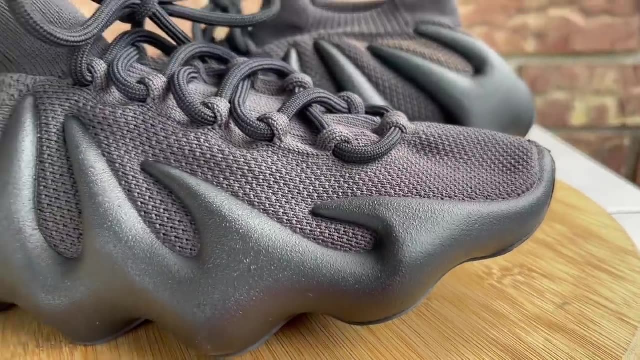 I'll upload something. So go ahead and hit the thumbs up. man, That goes a really long way. All right. So now that all that's out of the way, let's go ahead and dive into the review. So, like I mentioned, this is the Yeezy 450.. This is your dark slate colorway. We had that first. 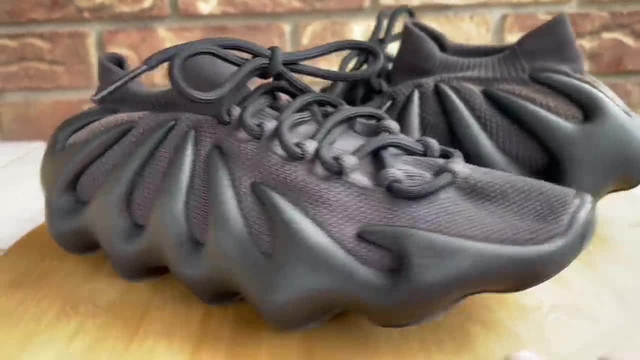 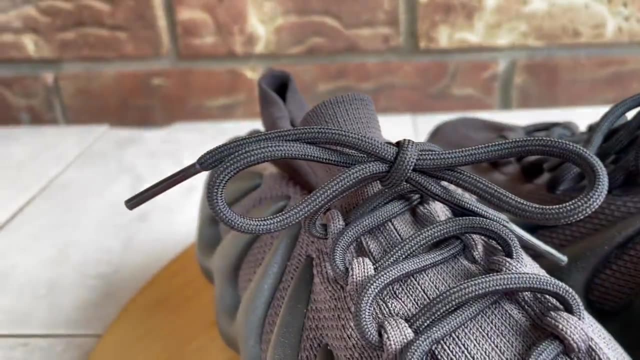 initial cloud white colorway that came out, And this is a silhouette that's either hit or miss, hate or love You either. I don't think there's anywhere you could be in between on this one, you know, like on the fence, I think. for this particular silhouette it's really out there. 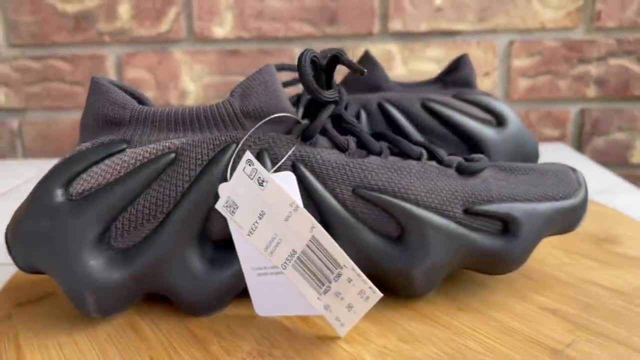 It's really weird and wild. I think you either love it all the way or you, like, completely hate it. It's not. it's not for you at all. I have the first colorway And I said: you know if they drop, like. 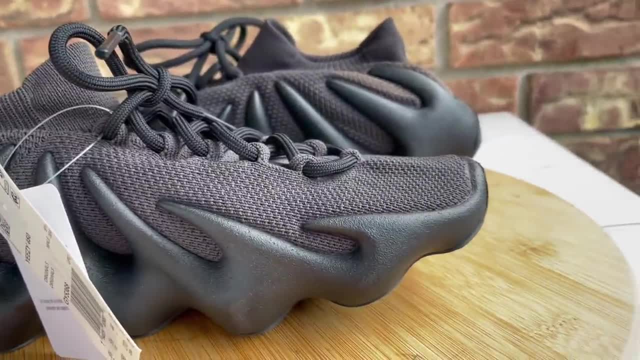 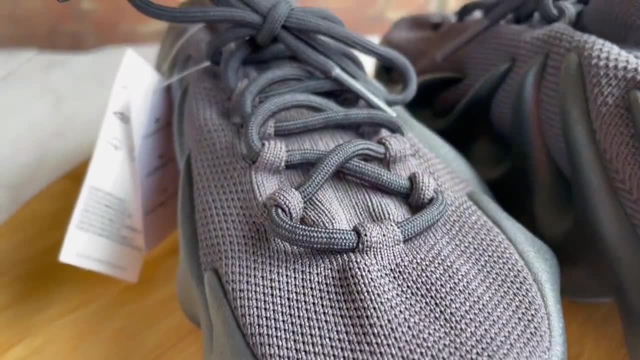 an all black colorway, something a little bit more, a little bit more darker. I would want to try those. And then, you know, these ended up releasing. So I'm glad I got these in the collection And this may be my last pair. I think I'm going to just be OK with just that first colorway. 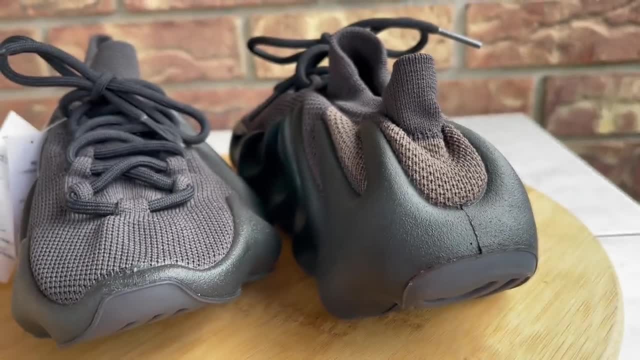 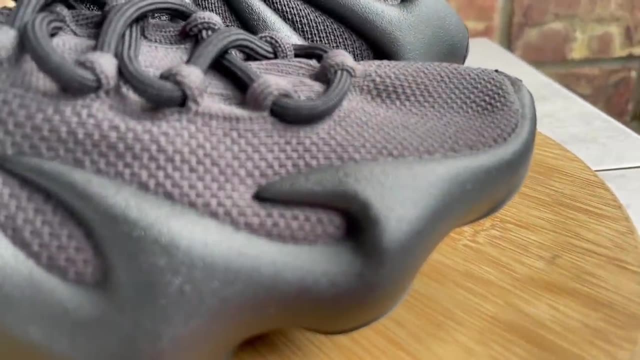 and then a black colorway, depending on what they end up doing, But this is definitely, you know, not for everyone It is. It's really out there A lot of pictures and comments. I get People say: it look like the dumplings. I get that emoji a lot whenever I post pictures of them or talk about. 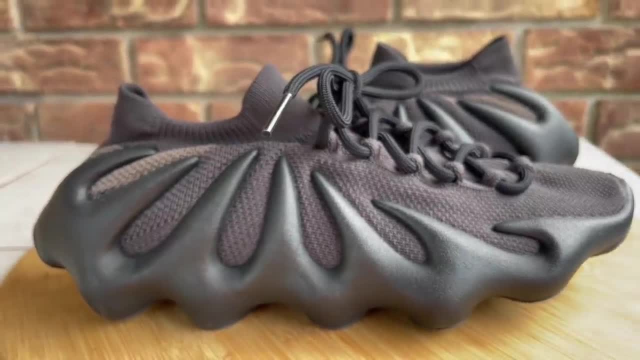 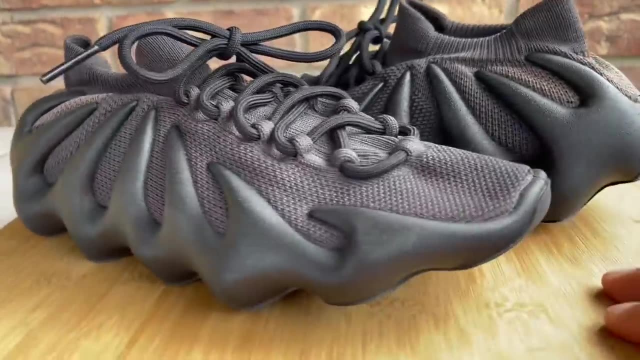 them, or whenever I read comments And it kind of does have like that little dumpling. look with it with these little claws down here. But it is it, Believe it or not, it's a comfortable shoe And I'm going to toss these on feet also, towards the end of the video I'm going to go over sizing. 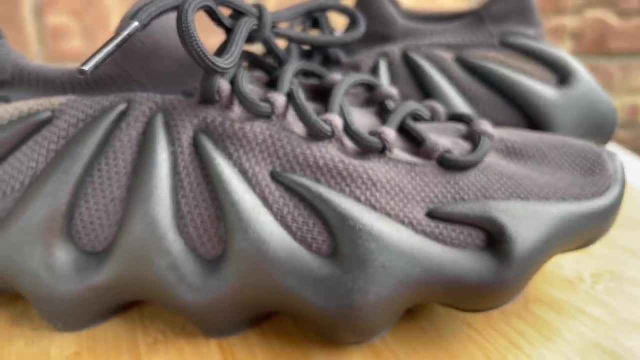 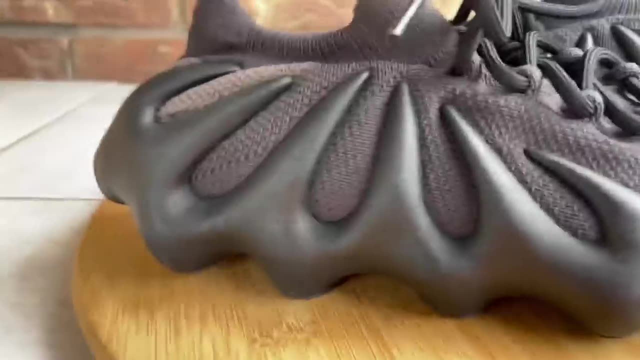 and comfort and all that stuff. But I want to give you guys a good look. I had the materials and everything that they used on the shoe first before I toss them on feet. So here you go, man. It's, it's really, really weird. You know it's, it's, it's a. it's a weird. 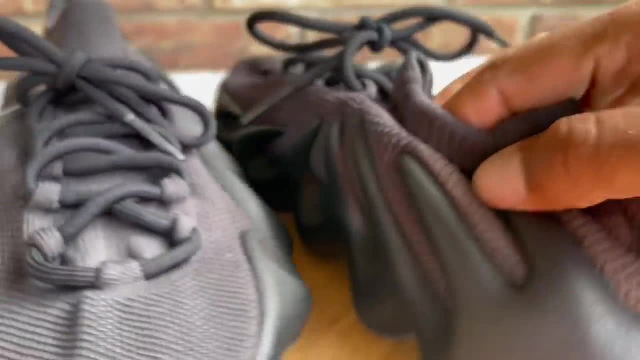 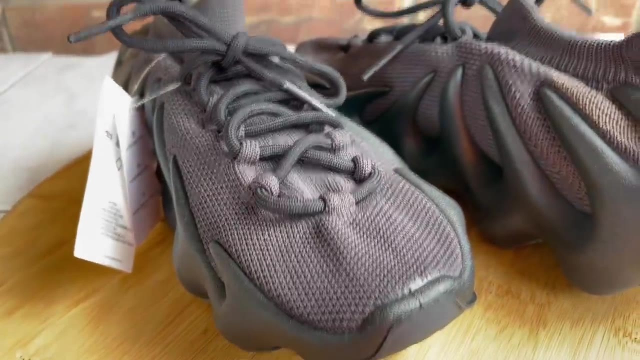 shoe And, like I said, I think you have to be one who's into, willing to try new things and, you know, not afraid to step out the box and try it, try something that looks a little bit odd, to appreciate these. You know, they're definitely not for everyone. 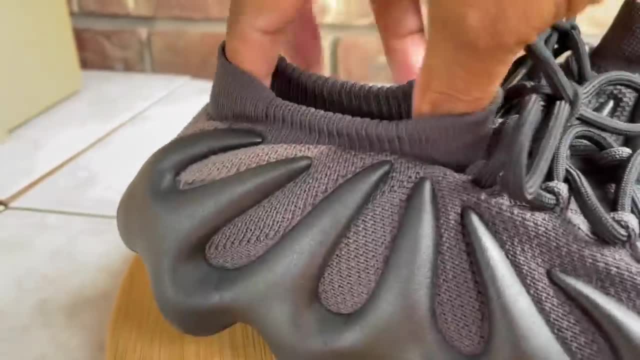 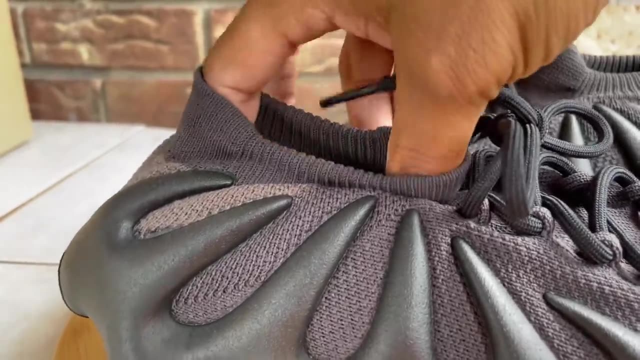 This sock little sock area right here where you put your foot in. You know, if you have like really really wide legs and fat feet and all that, it's going to be a challenge trying to get this on. It stretches, yes, But you know, initially it is, it's going to be a challenge to get it. 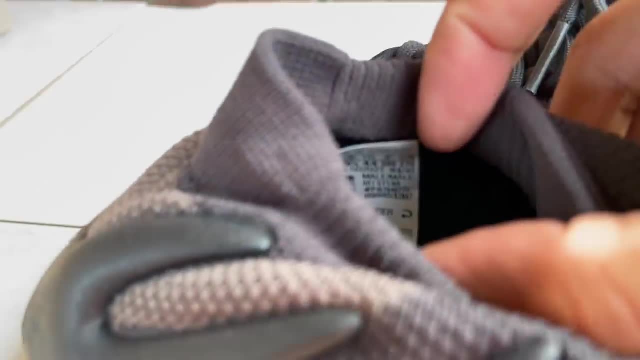 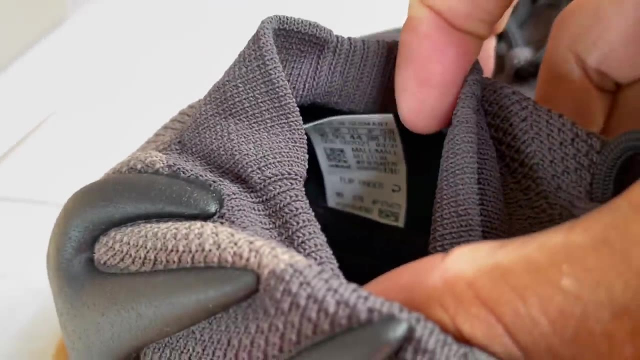 get it on. I have a medium to narrow width foot and I still have a little- you know a little- problem getting them on. I'm trying to get the label down in there for you guys So you guys just can see the production information and the label on here, But it's. 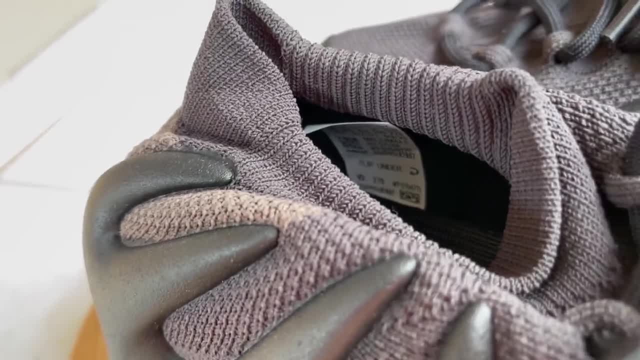 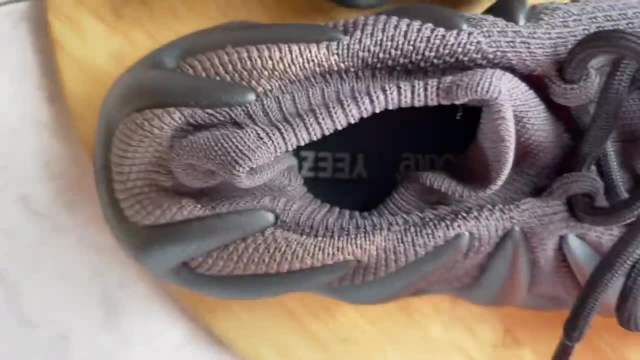 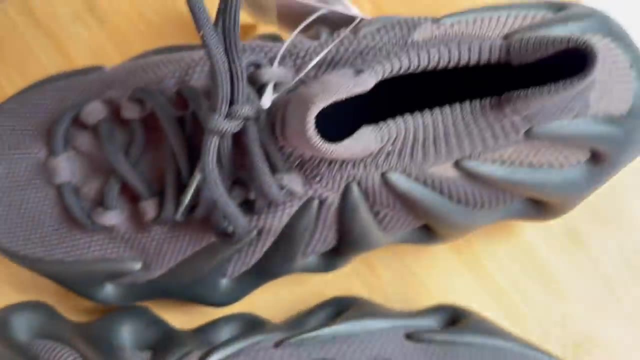 uh, you see, if I could zoom in on that for you guys, if you can get it, All right, I'll try and get it later. Here's the insole and that Yeezy insole- Some Yeezy branding. Look like it's an ortholite insole, like they've been using on a lot of the Yeezys that we have. 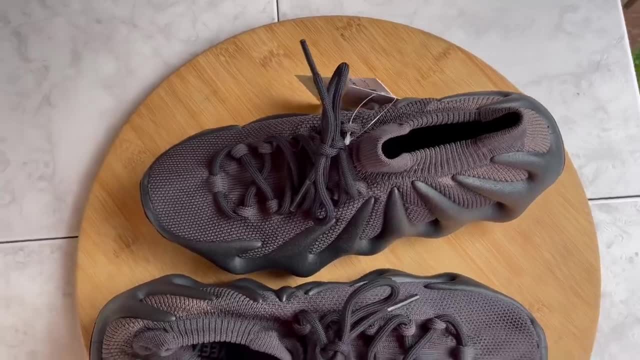 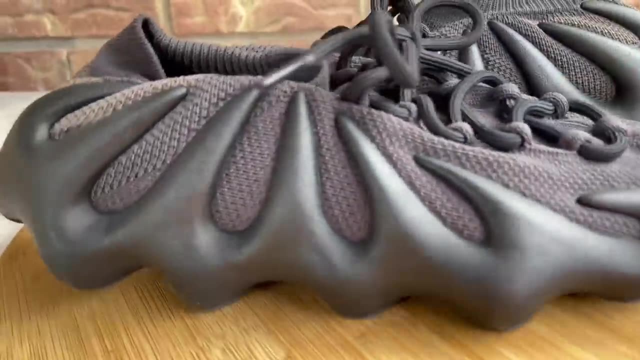 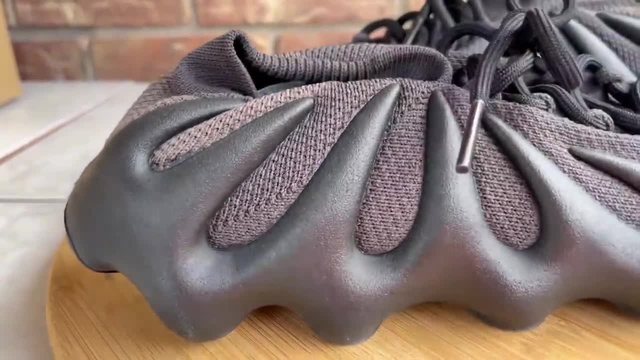 It's like a faded, ashy black color. It's like a faded, ashy black color. And then they lightened up the color towards the back, just like they did on the first colorway. I'm not. I'm not sure what's. 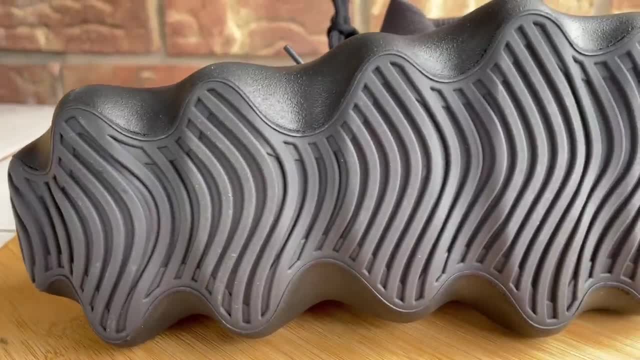 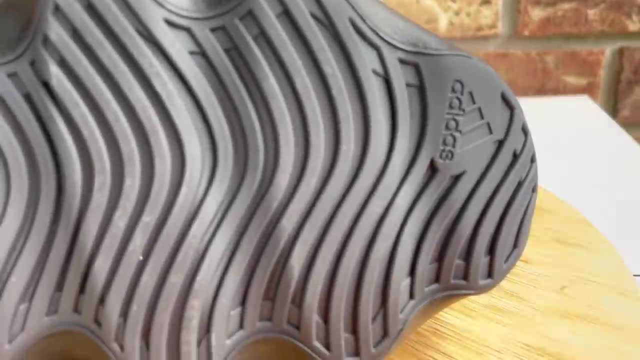 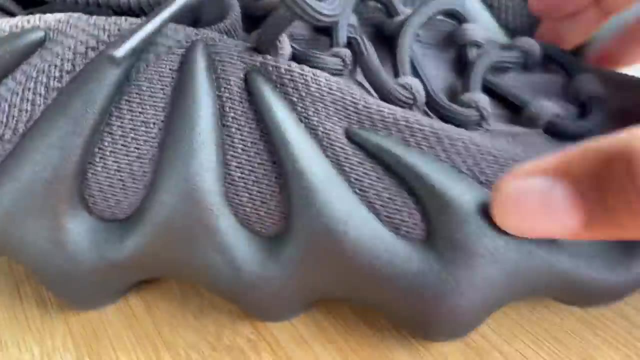 the intentions behind that, Like why they have a lighter color or a different colorway just towards the back of the shoe. Um, not really sure why Kanye and Adidas did that. So you have some Adidas branding right here also. Um, material wise. So this is like a foam, a hard foam, It's not. 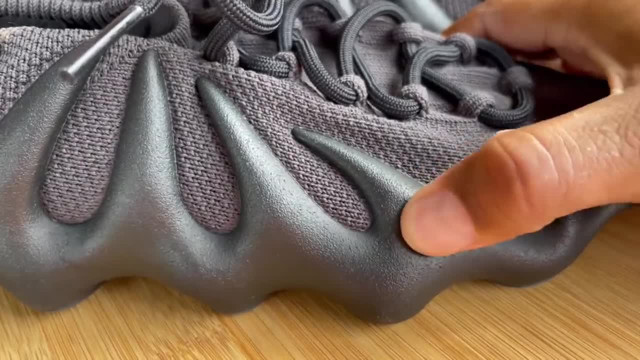 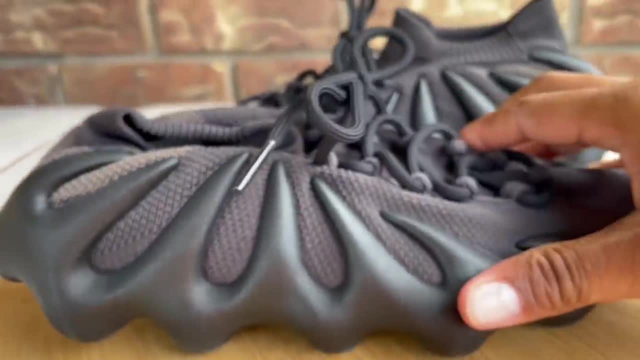 it's not squishy, Um, and it's not like rock hard It. it has like a you could push it a little bit, but it's definitely firm And I guess that's to you know, kind of support your foot, um, you know, while it's inside this, this sock type upper, I just primed it. 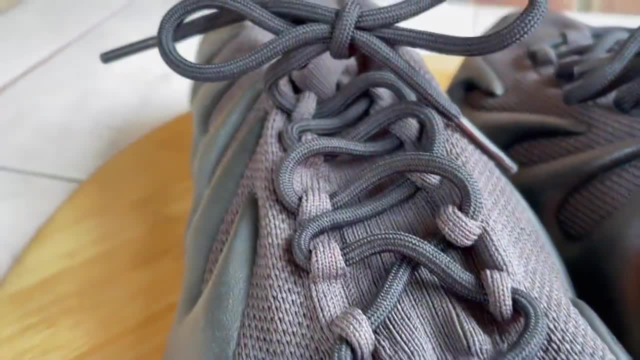 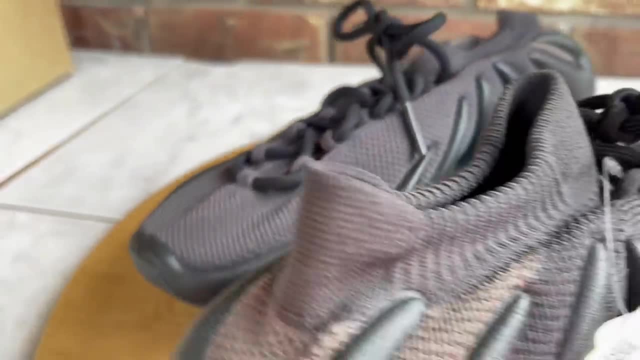 upper. You only get one set of laces. uh, and these are them, and you don't really need them cause you can't really tighten up the shoe or not. It just it's just like a really, really tight sock on your foot whenever you put these on. Uh, no extra laces, and they don't have the um like. 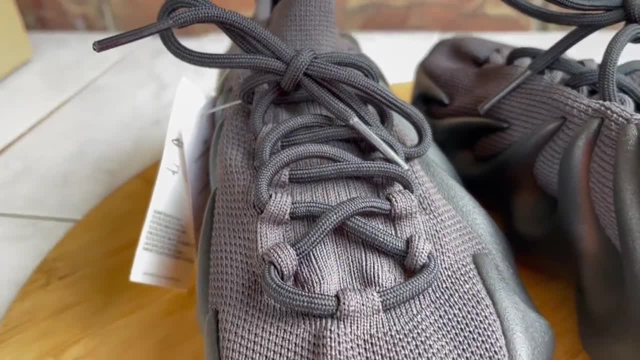 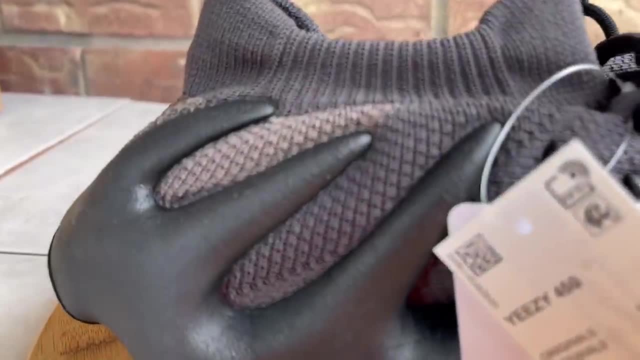 the infinity laces, And I'm glad they didn't, cause I'm not a huge fan of that infinity lace. Um so, here you go, man. Overall, I think these are. you know, I like odd shoes and anything that's going to draw attention to your feet whenever you wear it. Um so these are definitely. 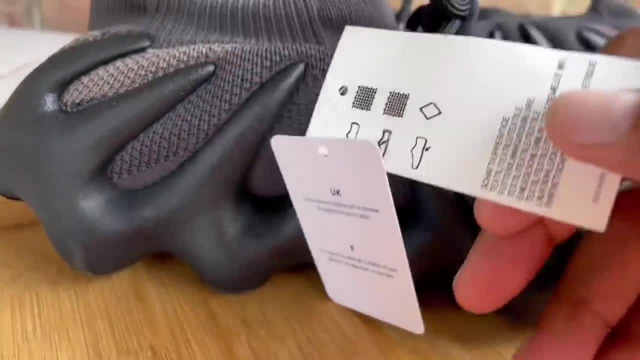 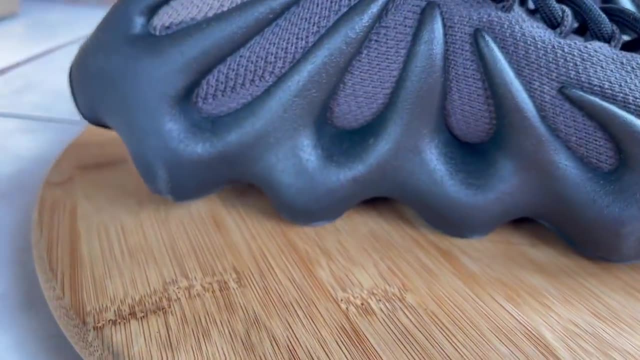 you know, something that I would buy and I would rock. So when I saw them I was like: all right, this is definitely up my alley, Let me go ahead and scoop them, add them to the collection. Um plus, I'm a Kanye fan also too. So, all right, here's the shoes. 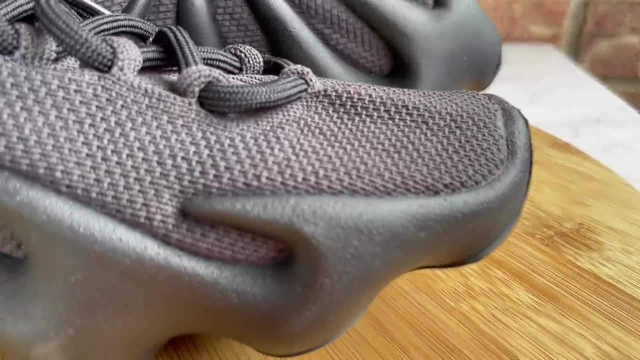 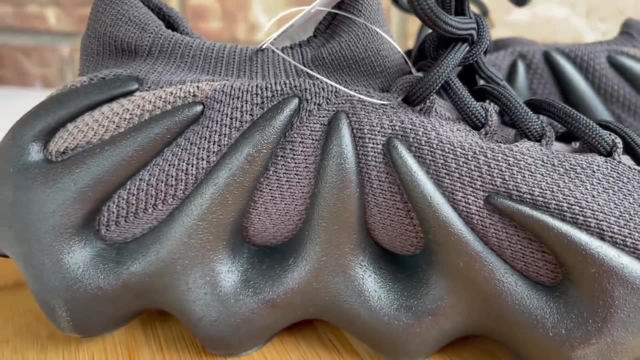 I'll show you guys one last look. Um, no real quality control issues. I don't really have any issues when it comes to quality control- um, in Adidas, not as much as I do when it like Nike and Jordan brand. So it did an okay job for its quality. you know nothing to really complain. 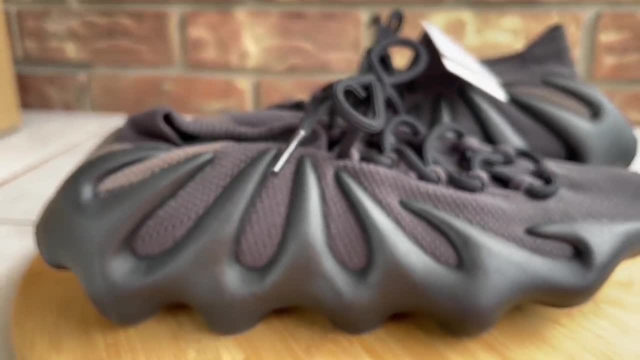 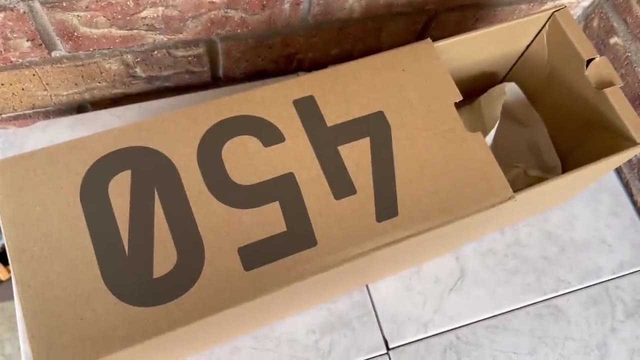 about when it. when it comes to these, Um, I'll show you guys the box really quick for a second before I toss them off feet. So you have a tiny style box, and that's just because you know. you know they're smaller than the actual slide box. The Yeezy slides box is larger than this. 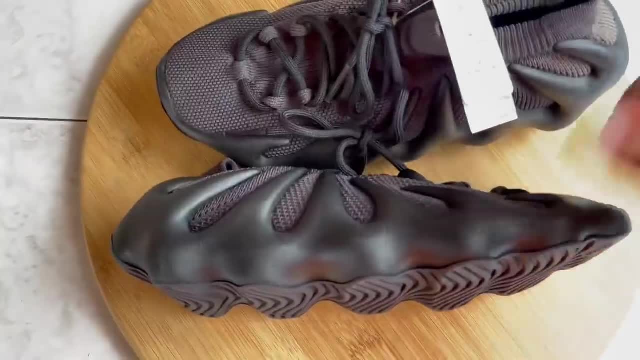 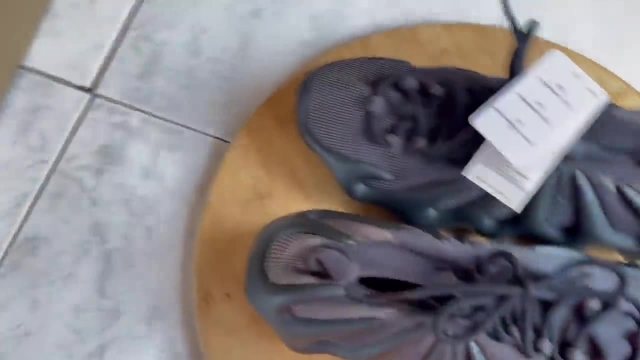 but you know it's like a pair of water shoes. So they came. you know kind of thin box like this So you don't really need a large size box to package these. So they were kind of just stuffed in this box. regular draw style box, no boost technology Cause normally. 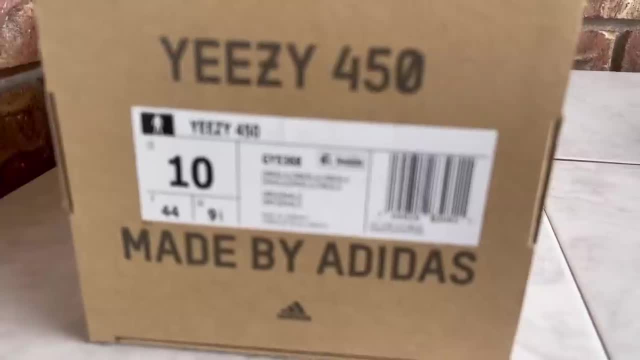 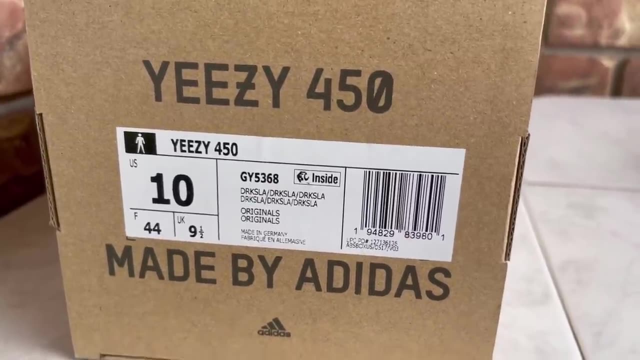 you would have boost written on a side. Here's your, your, your product code, your color breakdowns. have that dark slate, dark slate, dark slate. uh, Yeezy 450 on here And um, that's pretty much it. 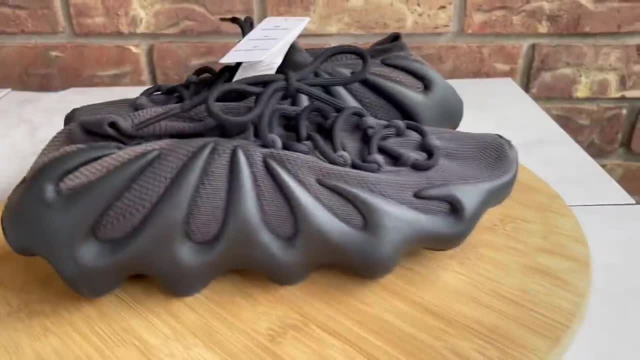 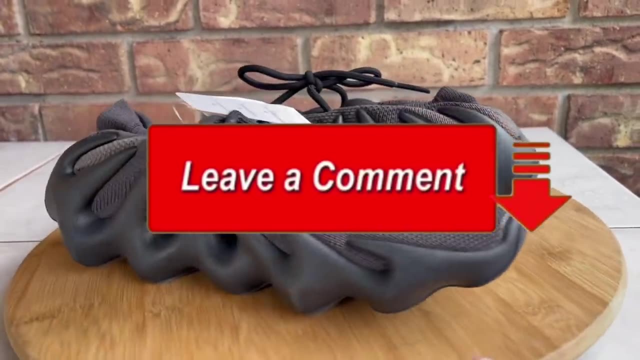 for the box. Show you guys the kicks one more time before I toss them off feet. You guys go comment. Let me know what you think of these. Let me know if you're a fan of them, If you like them. you hate them, Uh, would you rock them? I usually reply to you guys When you guys leave me comments. 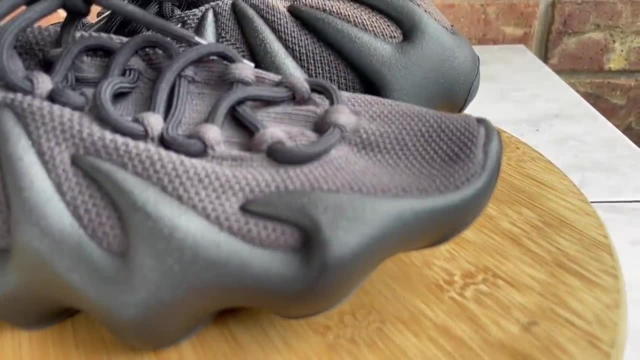 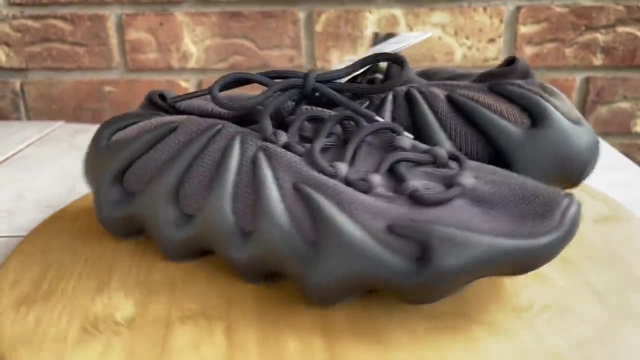 down at the bottom. If I don't reply like to directly what you said, I would hit the thumbs up or the heart button next to your comment just to interact with you guys in a comment section. Uh, so let's talk in the comment section. Curious to see what you think about these. 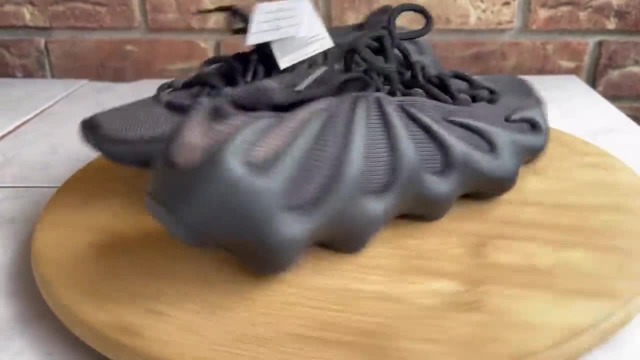 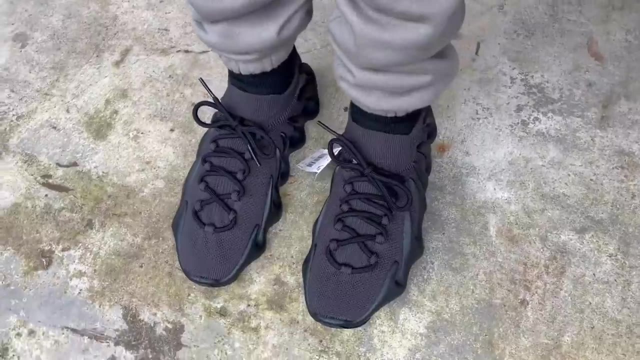 And, um, I'm gonna take them off him and toss them on feet. Let's see what they look like. All right, guys. So here's an on feet. Look at your dark slate Yeezy 450s. Just want to give you guys a quick look and show you what they look like on feet. 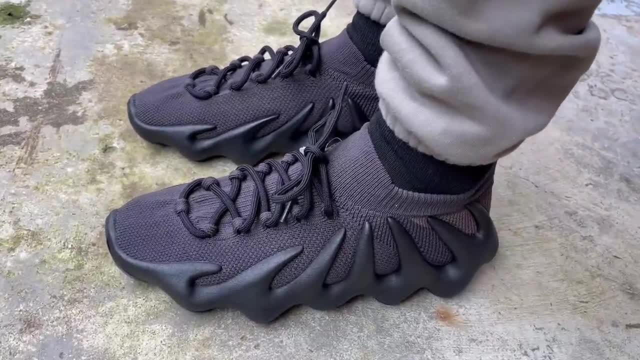 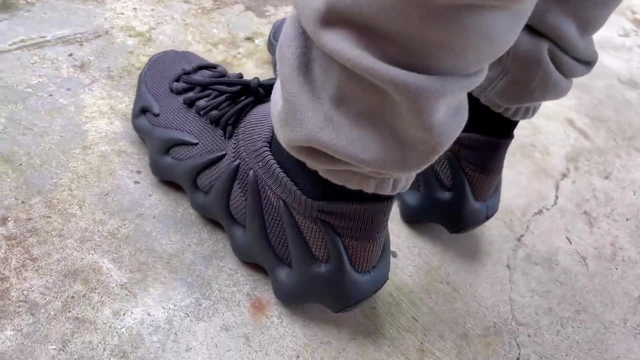 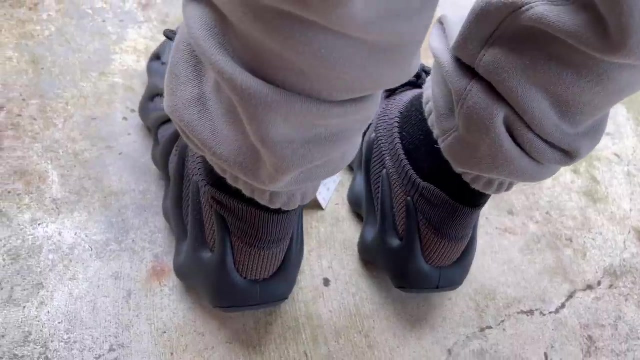 Uh, so the first things. first, and usually my my most asked question is size and how do these fit? How do they run? I have a medium to narrow width foot and I went true to size in them And the shoe fits really snug and exact like a really tight sock, If you don't like a tight. 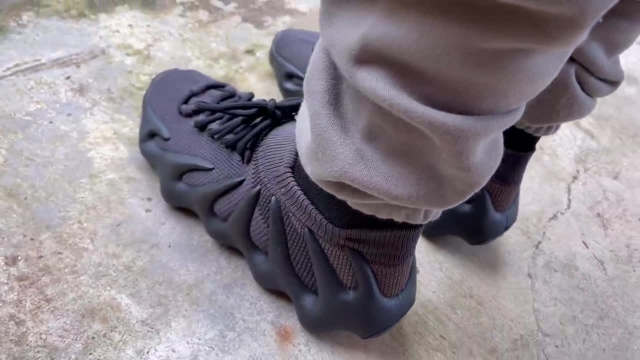 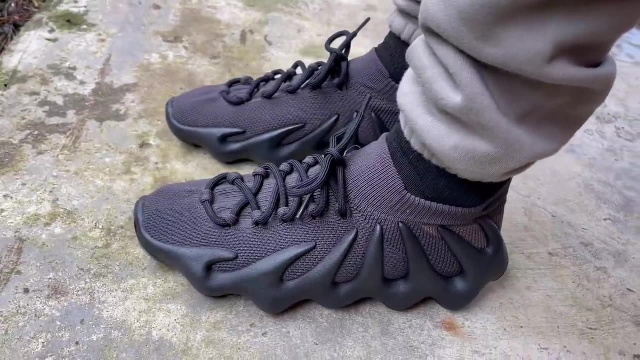 snug, exact fit. I would recommend going up a half size, Uh, but if you want that fit like I like, I think you'll be okay. And then, with the upper being made out of like a knit material, I think the more you wear them they'll eventually start to kind of break and give and start to feel. 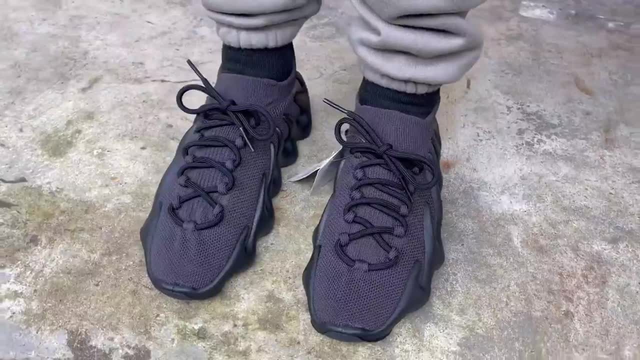 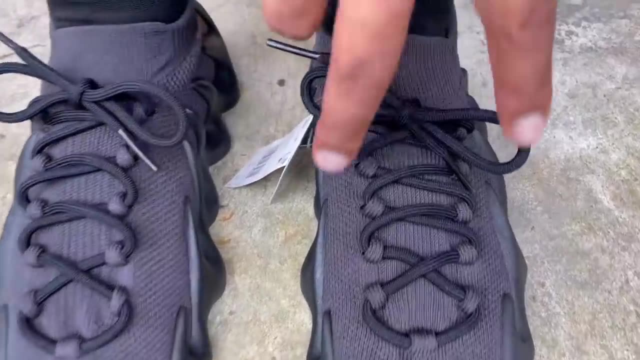 a little bit better. So I think you know it's all on preference and how you like the fit of your shoes. If you have wide feet, these are definitely going to be a challenge for you. Uh, cause the shoe is really really snug all along here, Cause, like I said, it's it's, it's a, it's a knit, and